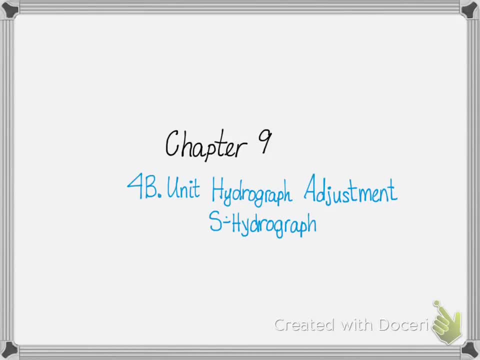 This video shows us how to construct an S-hydrograph and use it to create a new unit hydrograph for a specific storm duration. Thus, S-hydrographs allow us to generate an adjustment to an existing unit hydrograph. So what is a S-hydrograph? It's a summation hydrograph used to adjust the duration of a unit hydrograph. 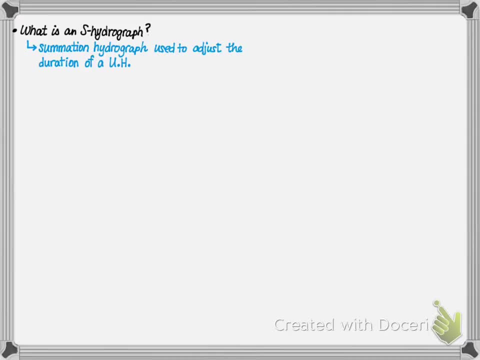 For example, if you have an existing one-hour hydrograph, we can convert it to a two-hour storm hydrograph. Or if you have a two-hour storm unit hydrograph, we can convert it to a one-hour storm unit hydrograph. How do you develop an S-hydrograph? First, you need to identify an effective storm duration. 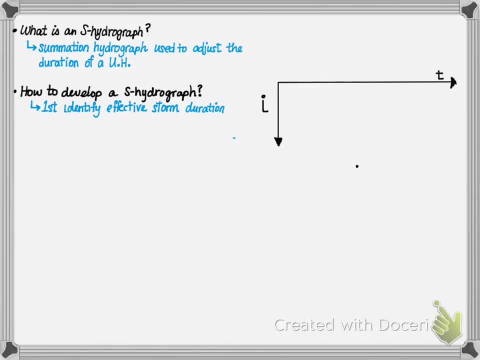 This is done by using an hydrograph. You're given a storm of duration t1 minutes. This is our effective duration. t1 could represent any time that we desire. Second, we obtain a specific unit hydrograph for a storm of t1 duration. 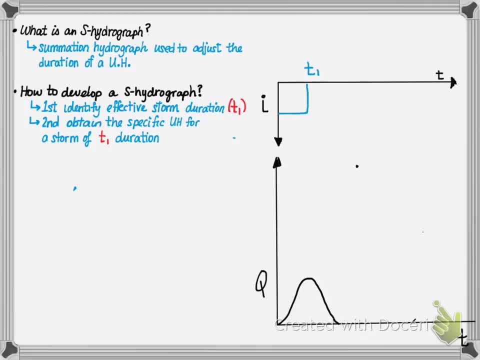 This unit hydrograph provides us a representation of a unit hydrograph for a duration of t1.. Next we repeat this unit hydrograph and effective rainfall: indefinitely. The start of the unit hydrograph is always at the same time as the start of the effective duration. 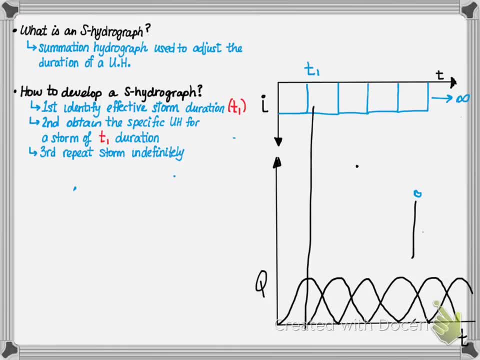 Thus you can see that they line up. Next, we need to sum up the unit hydrographs to develop an S-hydrograph. Thus there's our S-hydrograph. Let's do an example to demonstrate how we truly use an S-hydrograph. 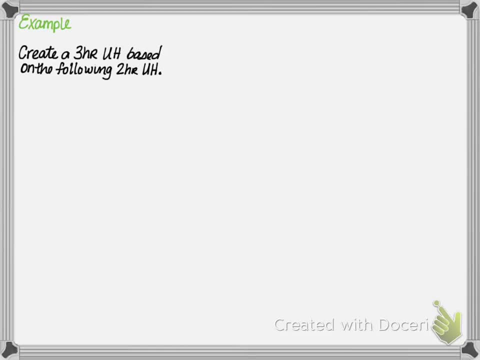 Create a 3-hour unit hydrograph based on the following: 2-hour unit hydrograph: These values are given to us every 2 hours over a 10-hour time period. The first thing you do is you repeat the unit hydrograph as described previously. 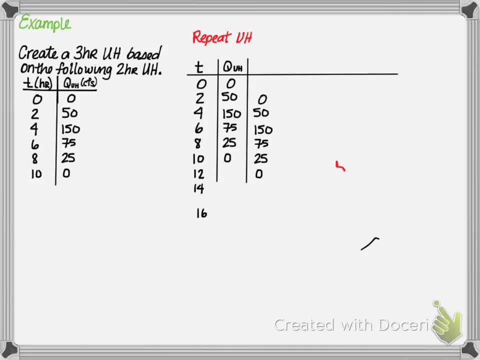 Since it's a 2-hour unit hydrograph. the 2 hours describes the effective storm duration, So every 2 hours we repeat the unit hydrograph as follows. Then you sum the values to construct the S-hydrograph. Once the value repeats itself, for example in this: 300,, 300, 300,. 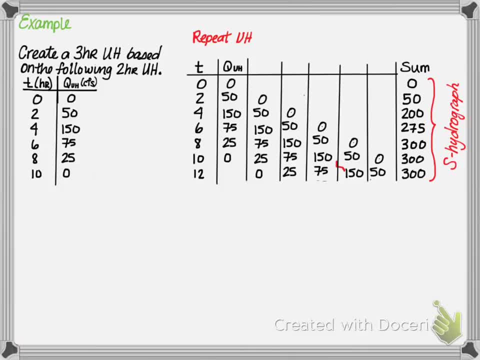 you know you have reached the plateau or top of the S-hydrograph And you no longer need to repeat. Now let's create the 3-hour unit hydrograph. Let's rewrite the 2-hour S-hydrograph that we determined above. 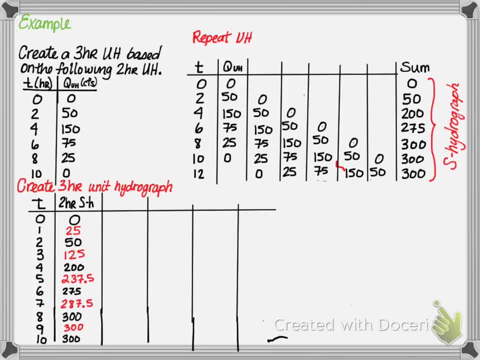 We need to interpolate between each of the 2 hours to find the 1-hour, the 3-hour, the 5-hour, the 7-hour and the 9-hour, Since we're constructing a 3-hour unit hydrograph. 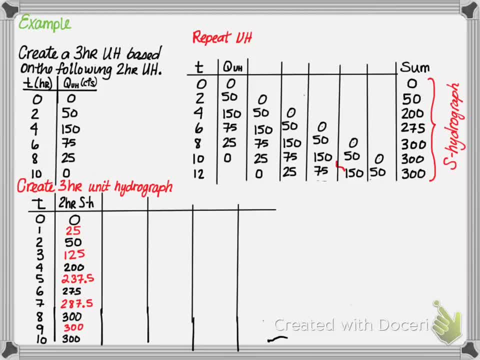 we did this simply by doing a linear interpolation. Since we are doing a 3-hour unit hydrograph. we take the S-hydrograph- the 2-hour S-hydrograph that we determined- and we shift it. So the 0 right here corresponds to the 0 at 3 hours. 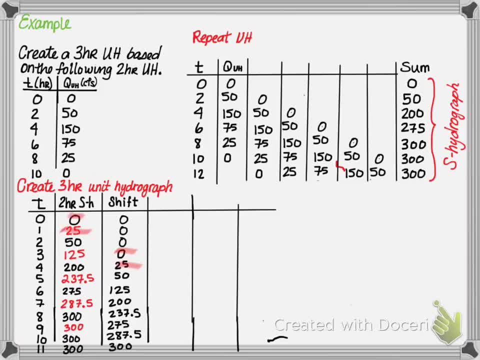 The 25 corresponds to the 25.. The 50 to the 50, and so on. Next, you take the difference between the 2-hour S-hydrograph with the shifted S-hydrograph. 0 minus 0 gives you 0.. 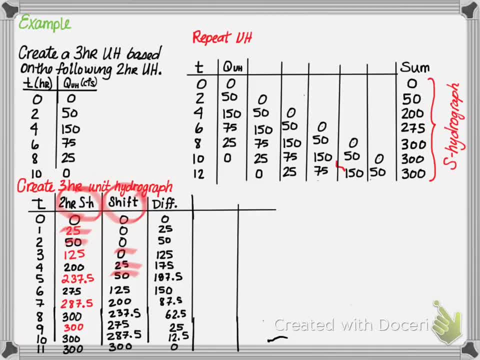 25 minus 0 gives you 25.. 50 minus 0 gives you 50.. 125 minus 0 gives you 125.. 200 minus 25 gives you 175.. And you repeat yourself. Next, you're going to calculate the 3-hour unit hydrograph. 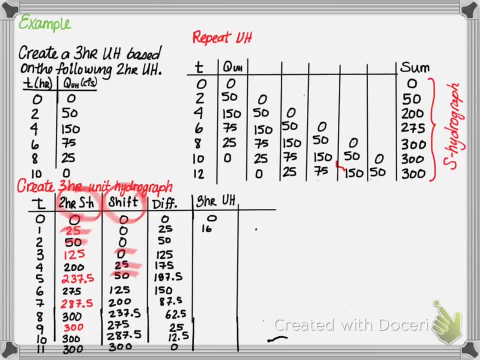 This is done by multiplying the difference column by the time of the original S-hydrograph or unit hydrograph and divide it by the new unit hydrograph. So in this case we will multiply each value in the difference column by 2-thirds.